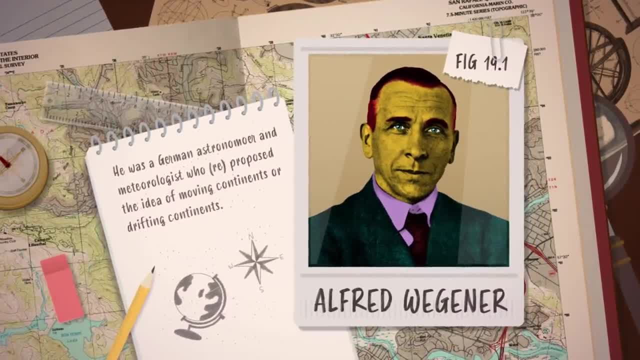 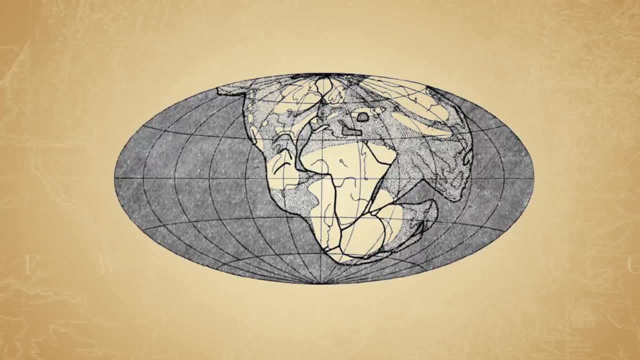 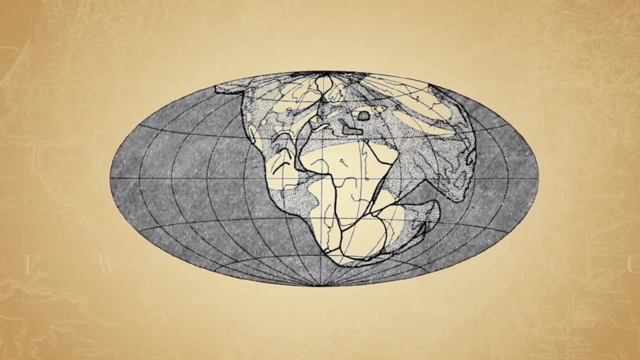 It would take over 300 years for astronomer and meteorologist Alfred Wegner to propose the idea again in 1912 and back it up with evidence Using the spatial distribution of fossils, location of rock types and trends of mountain ranges, among other evidence. he hypothesized that approximately 225 to 300 million years 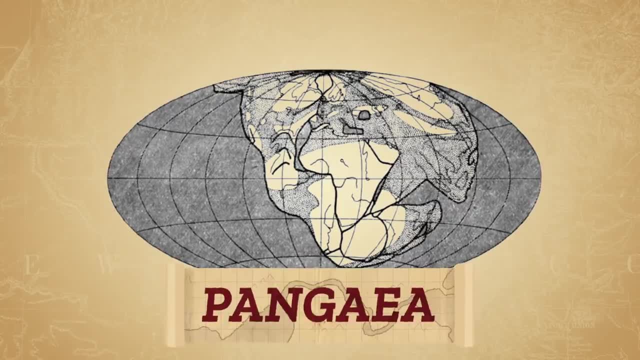 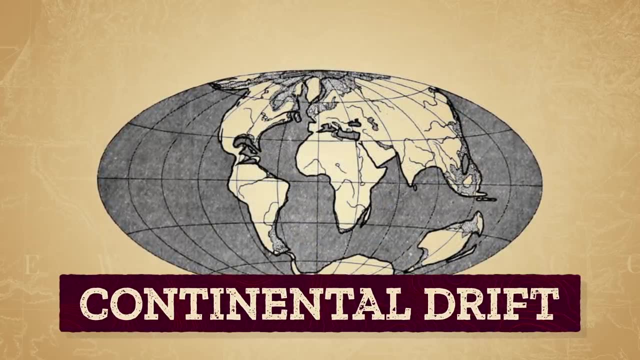 ago, the Earth's land was a single supercontinent called Pangea, meaning all Earth in Greek. It broke apart in a process called continental drift And eventually led to the landmass distribution we have now, Which was an outrageous proposal to the rest of the scientific community, Or you know. geologists who were upset that a non-geologist was horning in on their turf. And, to be fair, despite all his evidence, Wegner didn't have an explanation for the energy needed to break apart huge chunks of continents and plow them through the oceans. 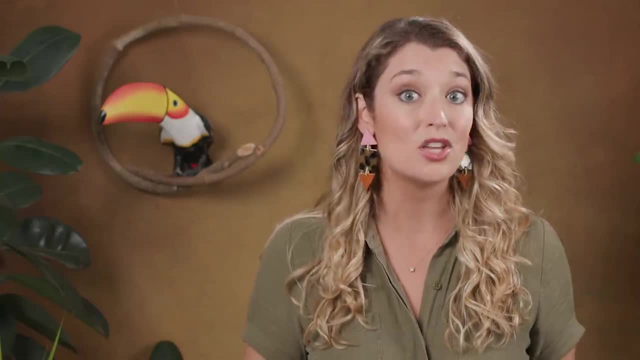 It wouldn't be until after the Second World War, when new evidence emerged from the depths of the oceans, that the idea of drifting continents was reactivated. In 1957, the first physiographic study of continental drift was published. It was published. 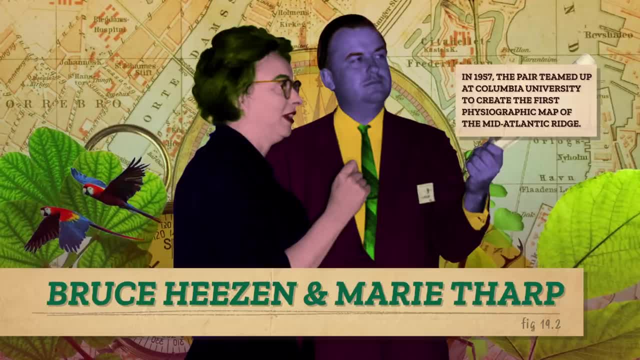 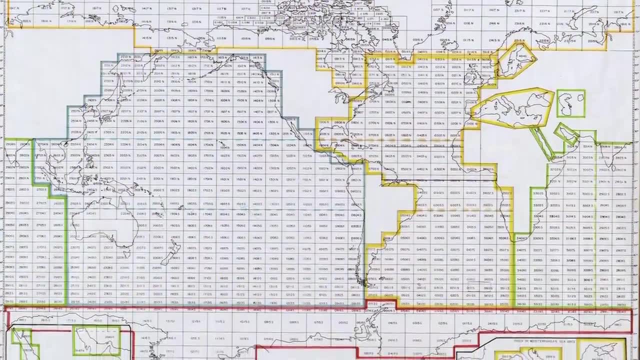 in the New York Times. The first biographic map showing the physical features of the Atlantic Ocean floor was published by two geologists, Bruce Heason and Marie Tharp. Using a type of sonar device called a continuous echo sounder, Heason collected bathymetric 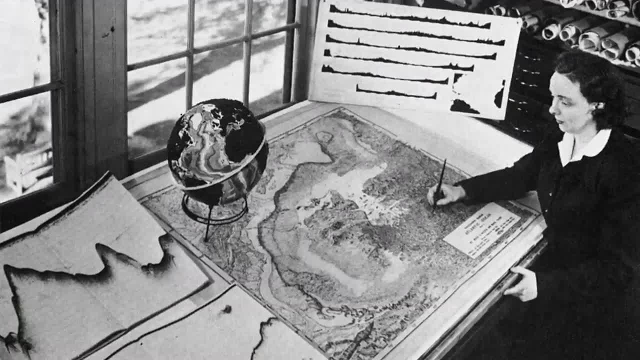 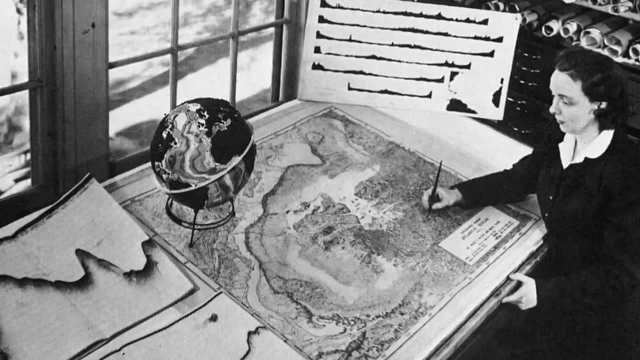 soundings, which are different depth measurements. This was the early 1950s and Tharp couldn't go on research expeditions because she was a woman, so she converted the raw data into maps that revealed how the ocean would look if drained of water. 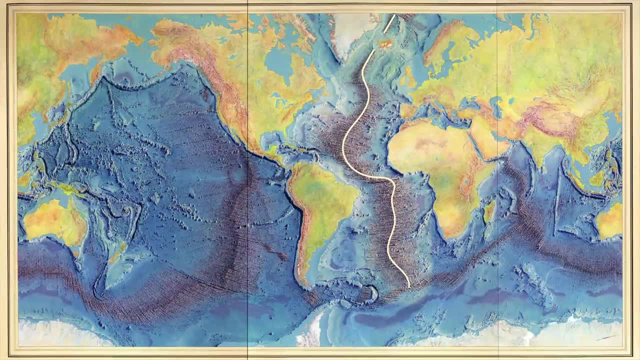 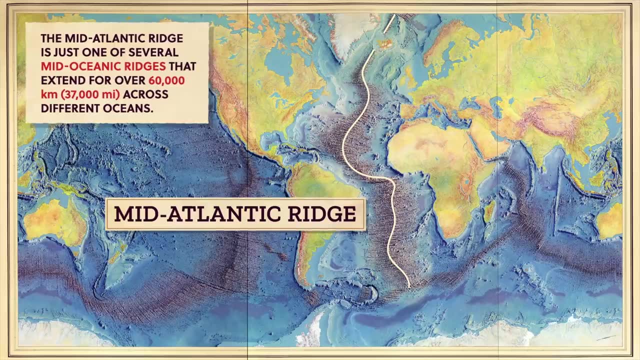 The centerpiece of their map was a vast mid-Atlantic mountain spine, criss-crossed by huge fracture lines called the Mid-Atlantic Range. Heason and Tharp focused first on the Atlantic, but it's just one of several mid-oceanic. 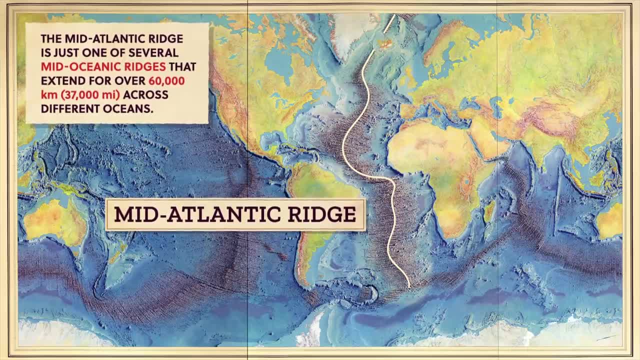 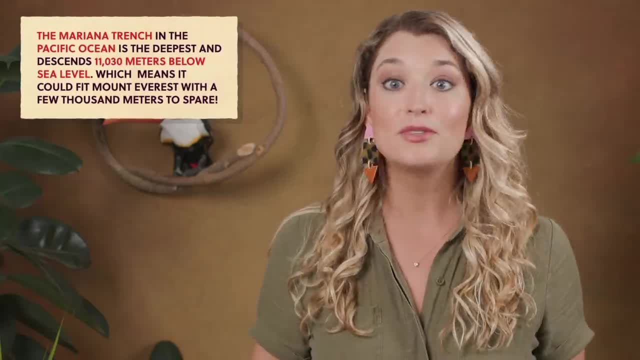 ridges that extend for over 60,000 kilometers across different oceans. Heason and Tharp changed how we thought about the Earth, because the ocean floor wasn't just a flat, featureless plain, like we'd assumed, but had mountains, valleys and even. 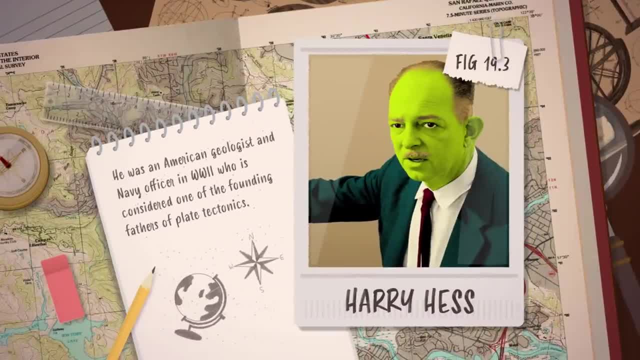 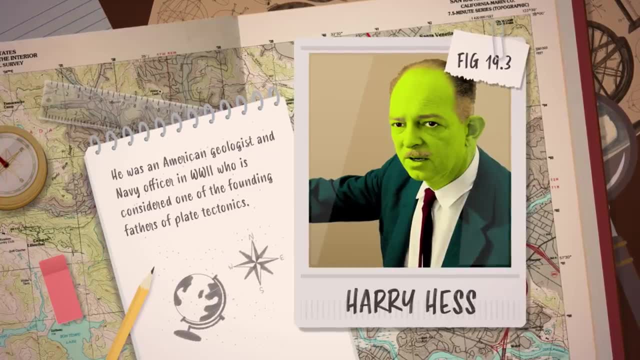 deep trenches, which are the deepest feature on the planet. Then, in 1960, Harry Hess, a geologist who had collected vast amounts of ocean data when he captained a ship equipped with an echo sounder during the Second World War, proposed that even more was happening on the seafloor. 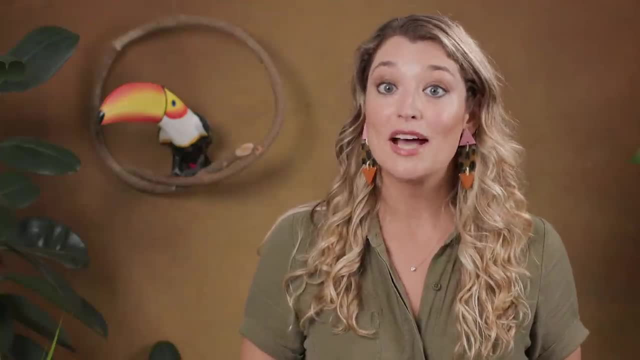 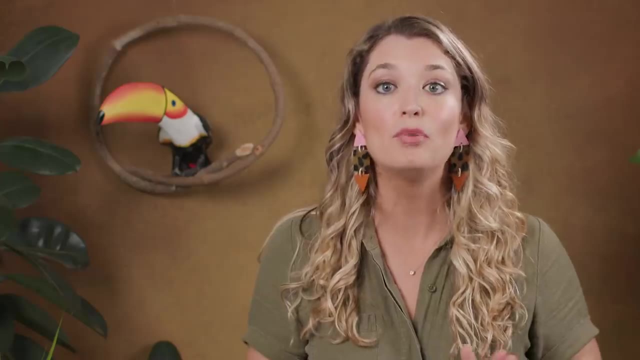 Magma spills out from the fracture lines of the mid-oceanic ridges, So Hess proposed that the seafloor was kind of like a giant conveyor belt. New seafloor was formed on either side of the ridges as magma flowed out and pushed. 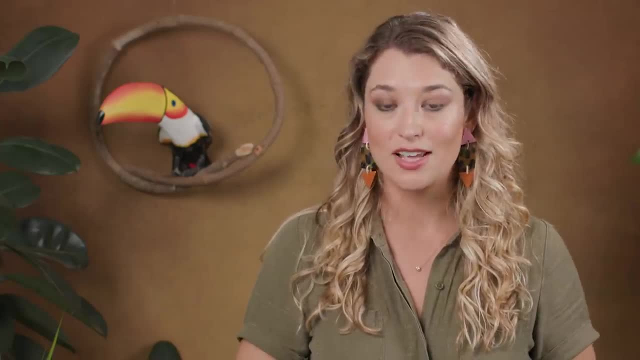 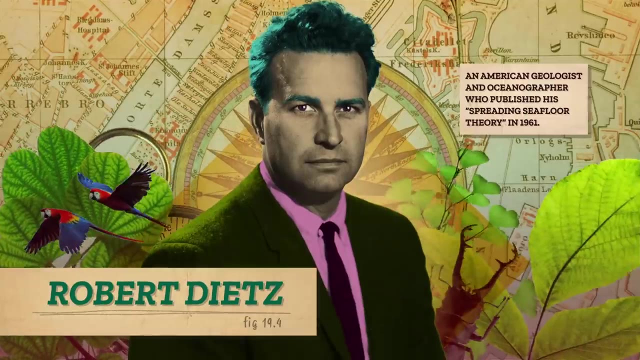 away the old seafloor And when it finally reached the distant trenches, the old ocean crust was cooled and dragged down into the mantle and recycled, Which was another radical theory, Though geologist and oceanographer Robert Dietz published a similar idea. he called the 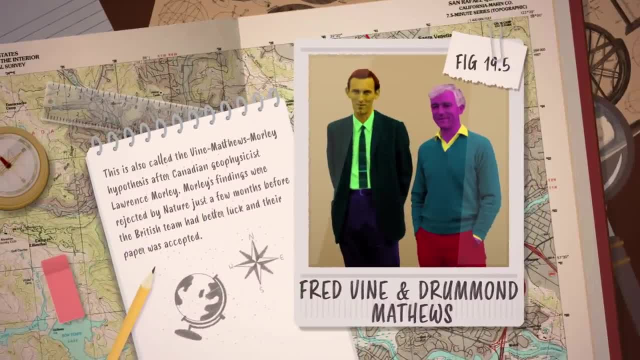 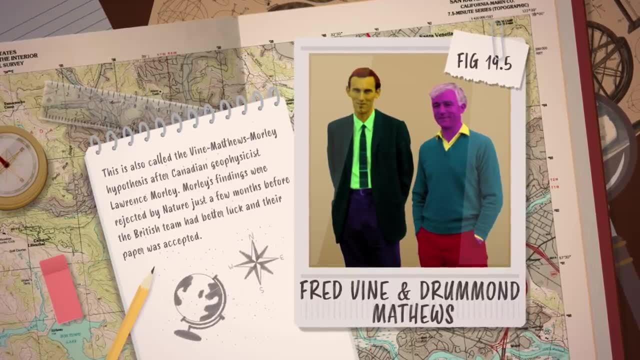 Spreading Seafloor Theory in 1961. But the evidence was actually recorded in the seafloor itself and published a few years later in 1963 by geologists and geophysicists Fred Vine and Drummond Matthews. You see, the Earth's magnetic field reverses periodically and this is recorded in rocks. 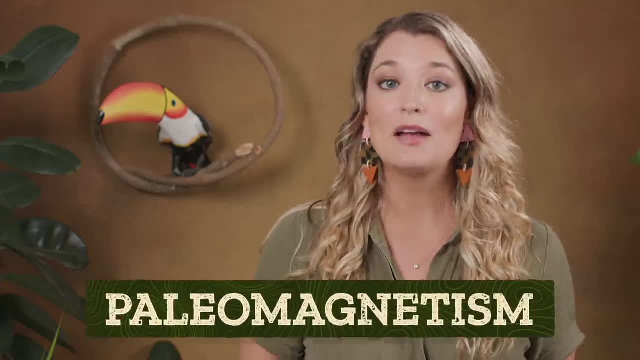 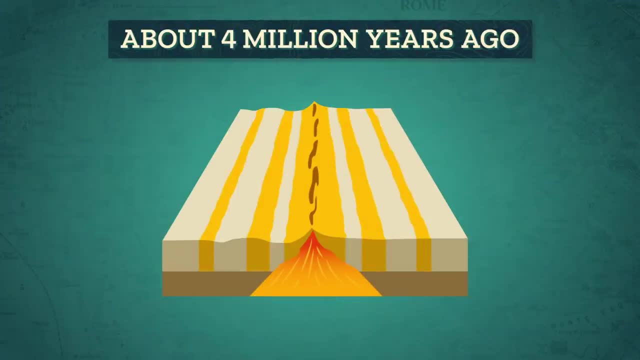 that contain iron as part of Earth's paleomagnetism. When magma cools and crystallizes, the alignment of the magnetic field is locked in place in the magnetic particles of the rocks. So each time the Earth's magnetic field flipped, the magma erupting at the mid-ocean. 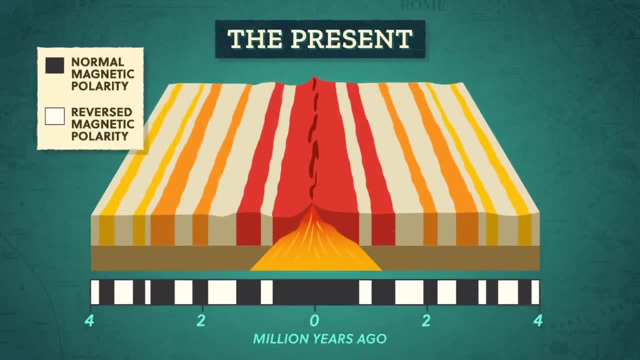 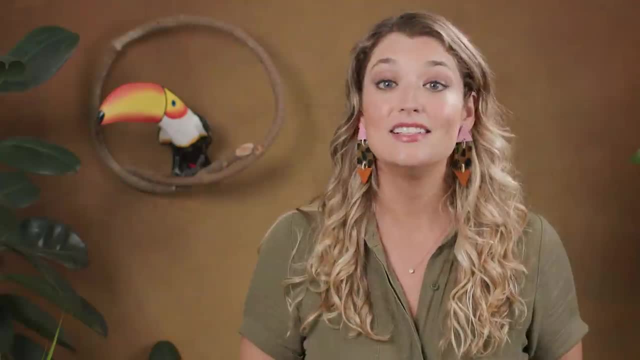 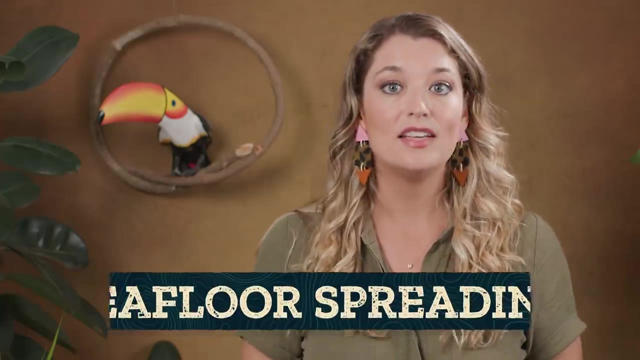 ridges recorded the opposite polarity to the previous batch. The result is a magnetic barcode of black and white stripes that mark where polarity changed, arranged symmetrically around the ridge. That means Hess and Dietz were really on to something And mid-oceanic ridges were built as magma on either side spilled out and spread laterally. 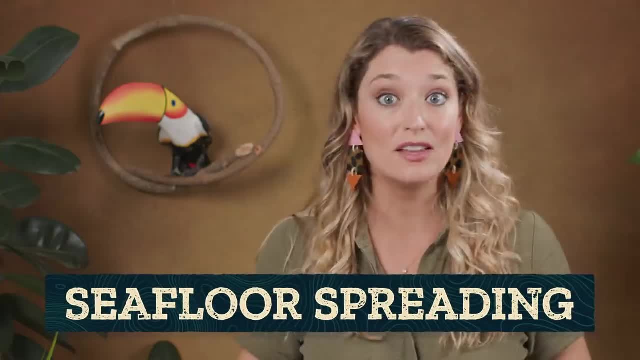 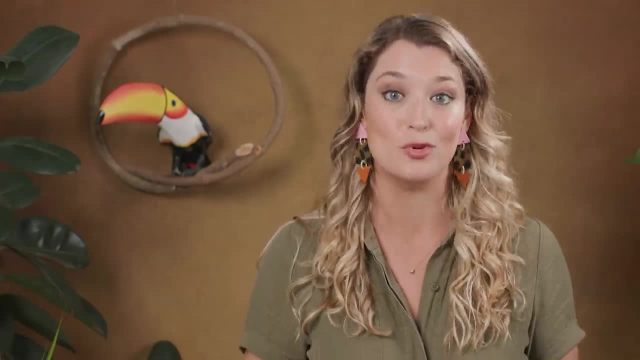 This seafloor spreading pushes the seafloor away in both directions and with it the Earth's landmasses, Which meant we finally had the evidence- Wegener was missing in 1912- for how the Earth's landmasses were moving. 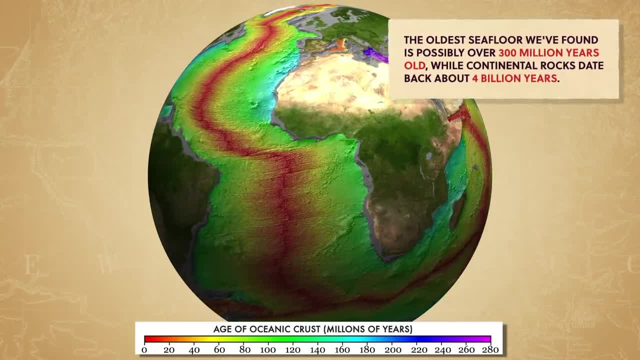 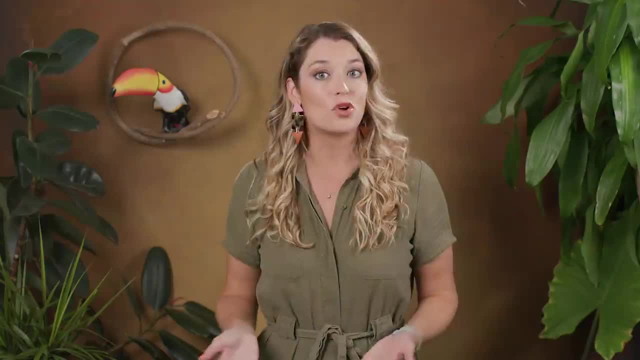 Thanks to seafloor spreading, all of the Earth's seafloors are quite young For rocks. In fact, determining the age of a basalt rock in the seafloor confirmed the matching patterns of magnetic histories. As for the crust being destroyed in the vast ocean trenches, it turns out that's exactly. what happens too. In the late 50s and early 60s, during the Cold War, when nuclear test bands were being negotiated between the USA and the USSR, a global seismic surveillance system was created to monitor underground blasts, Which also happened to provide North American seismologists with observations of deep earthquakes. 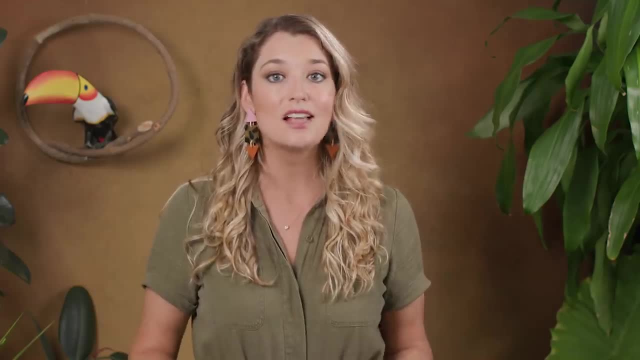 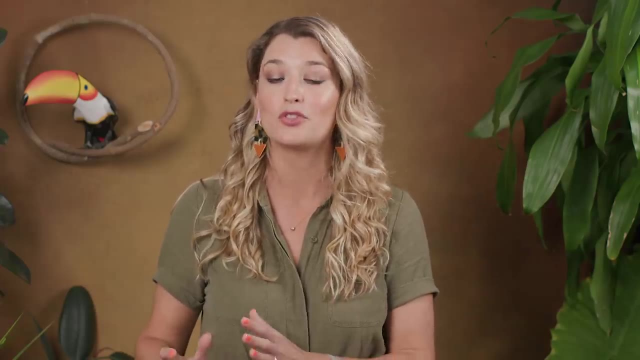 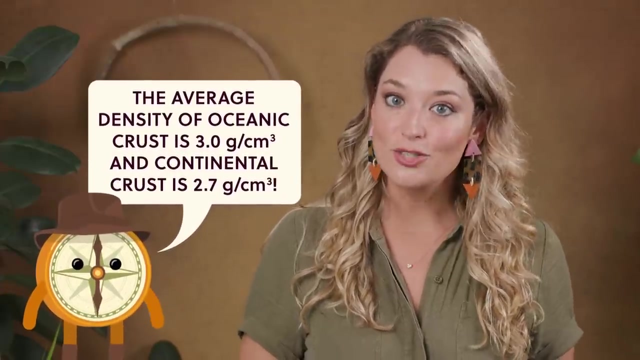 more than 700 kilometers beneath ocean trenches. These observations were later used to visualize a thick slab of Pacific Ocean floor that was being pushed under the edge of a different slab of Earth's crust and consumed into the mantle in a process called subduction. Because the oceanic crust has a greater density than the continental crust, the thinner, denser. 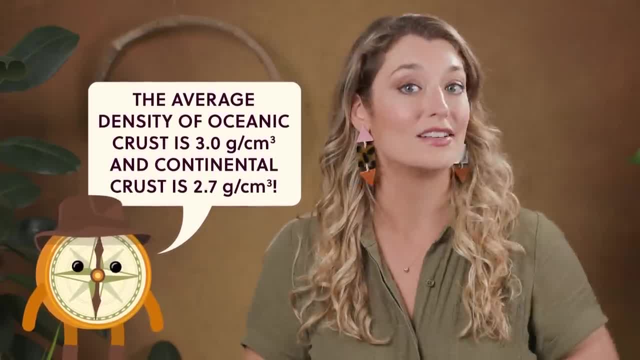 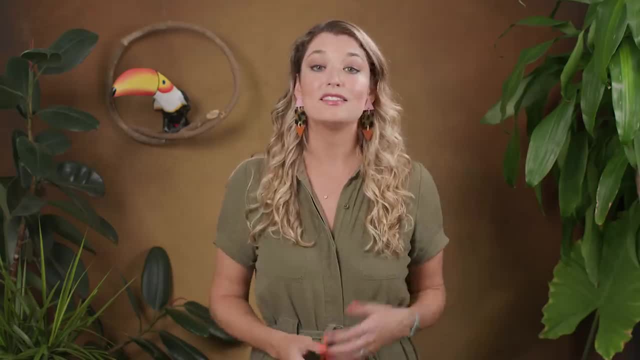 oceanic plate dives beneath the lighter, thicker and more buoyant continental crust, This forms a subduction zone And what we see on the surface is a giant trench. So, with ocean mapping, seafloor spreading paleomagnetism and crust subduction becoming 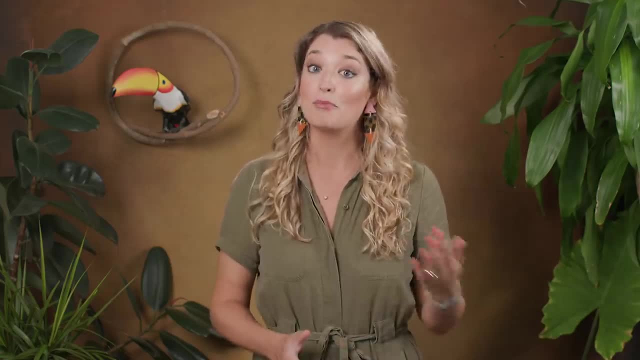 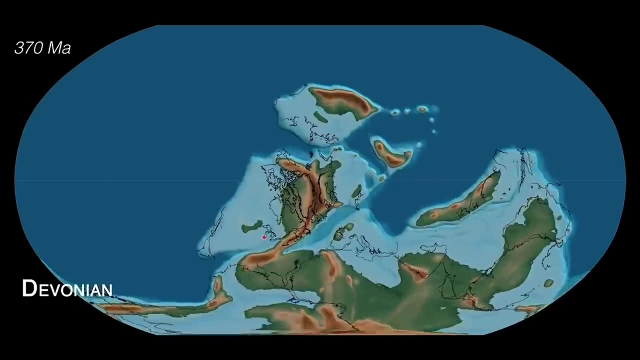 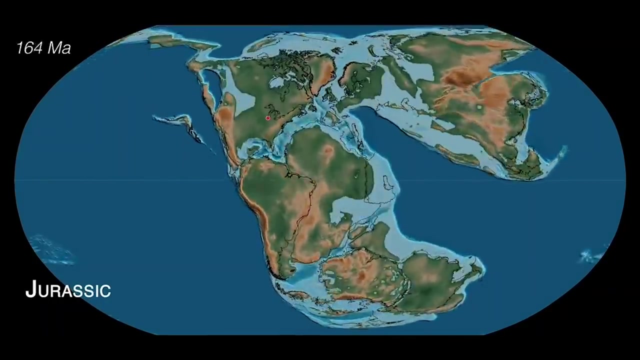 confirmed pieces of scientific knowledge. the world was now on the brink of a revolution. The final piece of evidence needed to produce a grand, unifying theory of Earth science came from precise mathematical calculations combined with new computing power. With these techniques, geophysicists were able to calculate how the coastlines of the 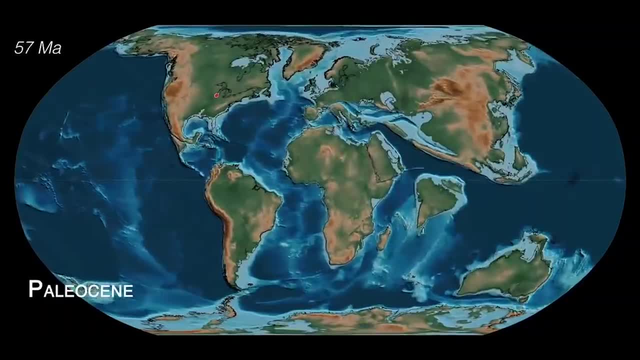 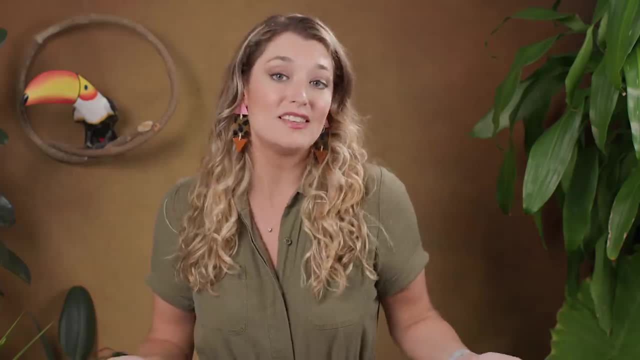 Americas, Africa and Europe best fit together and predict how the tectonic plates moved And with that a revolution unfolded in Earth science. Leading the charge was a bunch of mostly young, unknown scientists working in a history of geosciences. 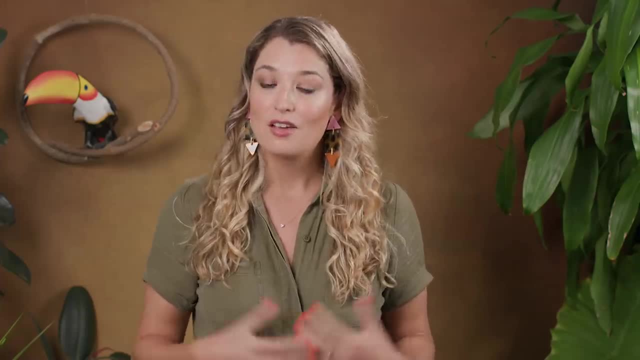 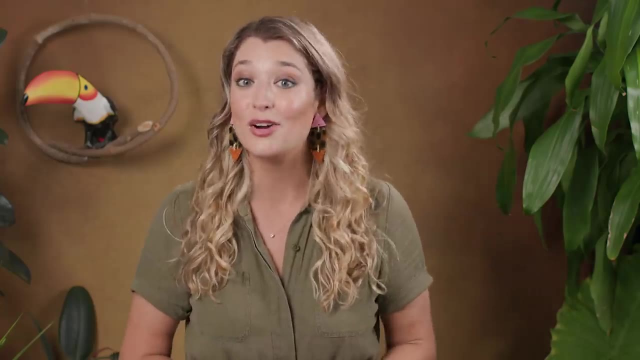 They were able to find a handful of institutions in North America, Britain and Europe. Fueled by the technology, money and military in those places, they peered into the depths of the oceans and fundamentally changed the way we understand the Earth. 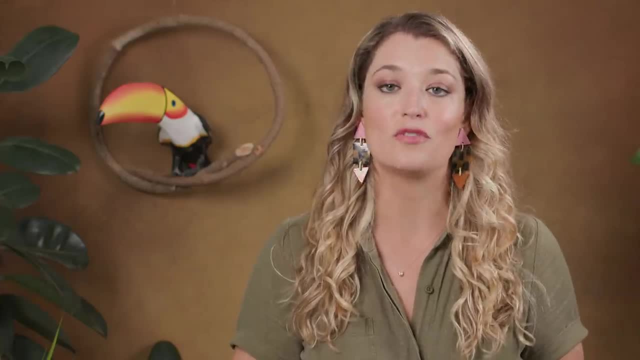 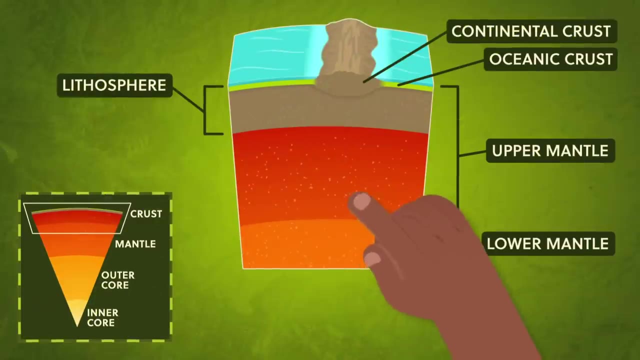 Years of independent research and disparate discoveries finally described the structure of the Earth's surface and led to a map of the world divided into moving plates, and created the theory of plate tectonics, Moving on average as fast as our fingernails grow the seven major plates and a scattering 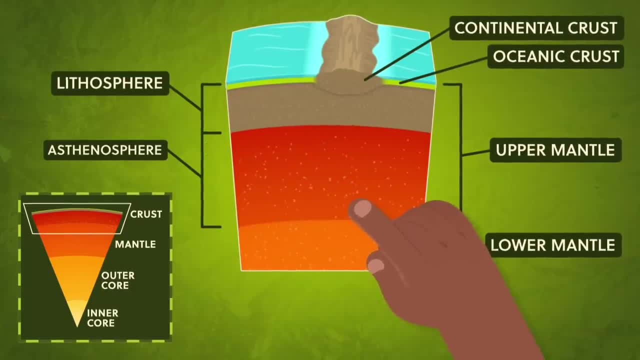 of microplates glide across the weaker, hot plasticky section of the Earth's surface. This is called the geosciences of the Earth, The geosciences of the Earth, The geosciences of the mantle, called the asthenosphere. 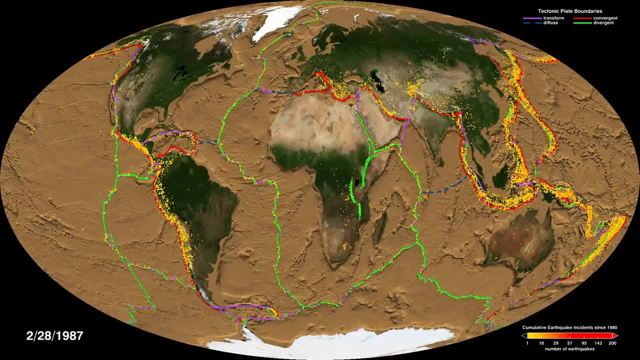 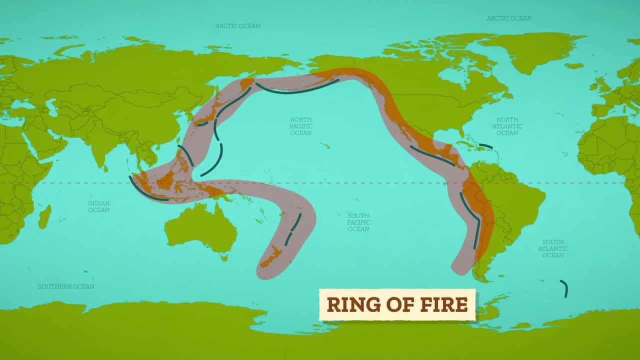 And we know now that where these plates meet are dynamic places where much of the planet's geological action happens, like earthquakes and volcanic activity, Like the area surrounding the basin of the Pacific Ocean is known as the Pacific Ring of Fire or the Circum-Pacific Belt, because approximately 75% of all volcanoes are dotted. 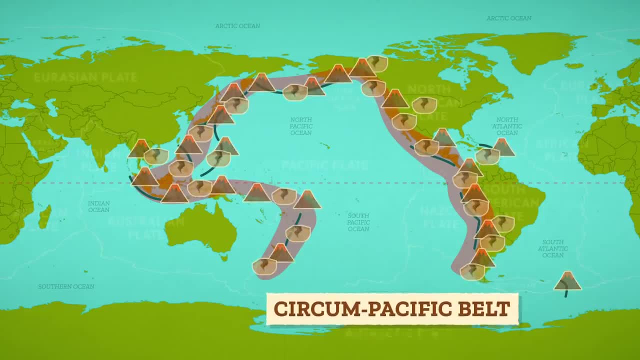 around it and 90% of earthquakes occur along its path. At the edges of the Ring of Fire, the plates come together in three different types of boundaries. On the eastern side, the seafloor spreads from the mid-ocean ridge called the Euclidian. 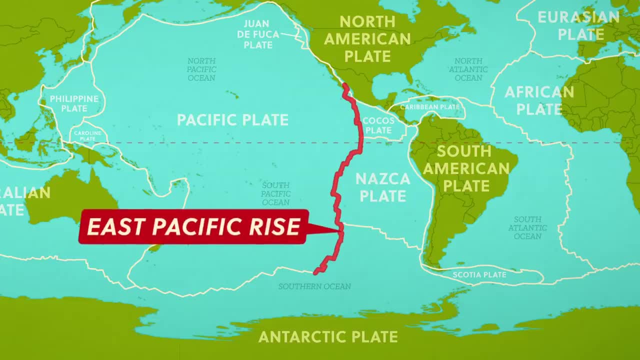 The Euclidian is the largest ocean in the world. The Euclidian is the largest ocean in the world. It's called the East Pacific Rise. that runs along the eastern edge of the Pacific Plate from near Antarctica all the way to North America. 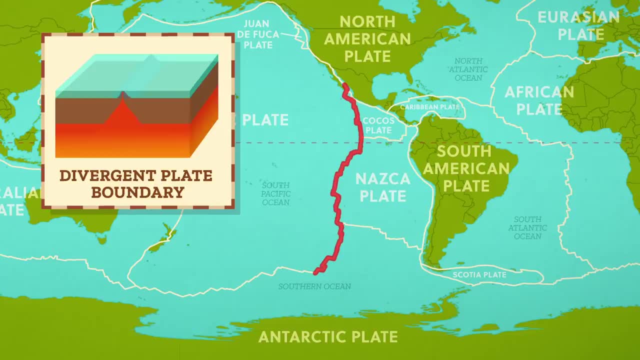 It's a divergent plate, boundary or place where plates are moving away from each other, with the Nazca Plate moving east and the Pacific Plate moving northwest. Along divergent plates, magma can well up and the seafloor regenerates and spreads. 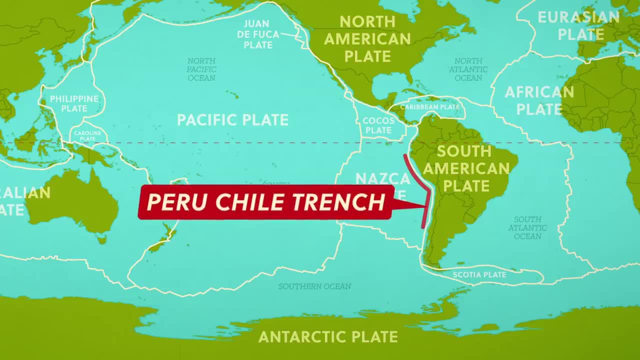 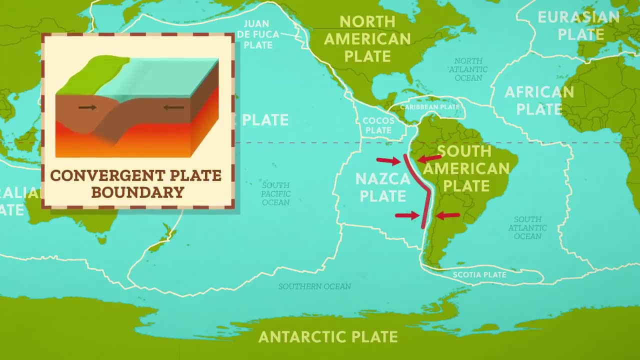 But farther south and west of South America. the Peru-Chile Trench marks the subduction zone where the denser oceanic Nazca Plate collides with and is pulled beneath the lighter continental South American Plate, Creating a convergent plate boundary. As the Nazca Plate is dragged down, enormous friction produces major earthquakes and hundreds. 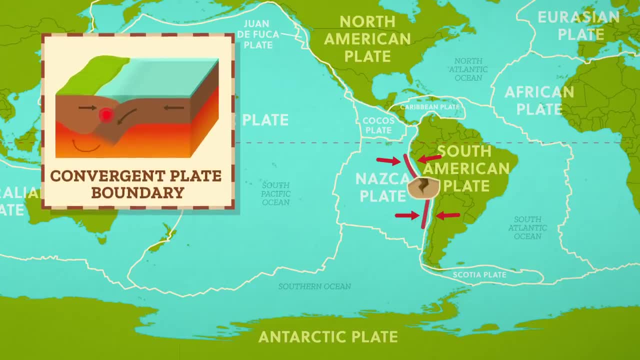 of meters of sediments are carried down into the deep trenches. As the sediments melt, they turn into magma which migrates up into the overriding plate And, where it reaches the surface, we get a volcano, Like the Andes, formed from plates colliding along a convergent plate boundary and have 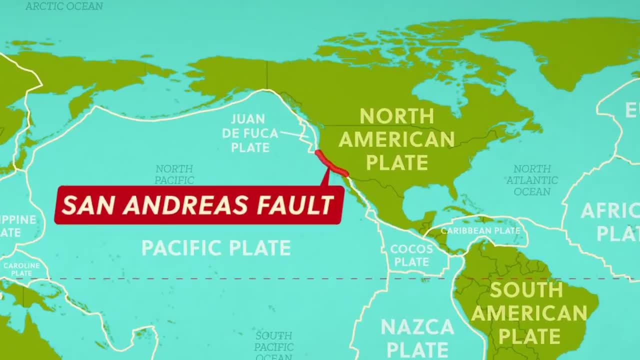 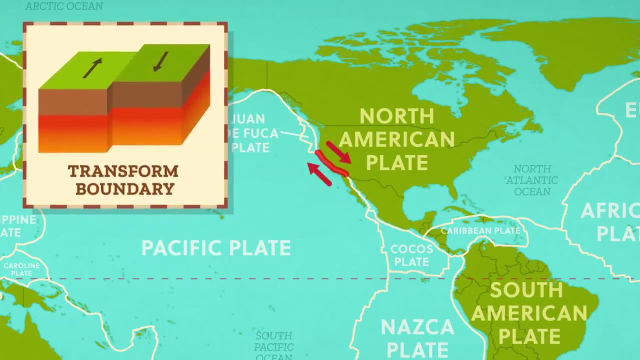 many volcanoes. Then, circling north again, we find the San Andreas Fault along the west coast of North America. It lies on a transform boundary where the North American Plate, moving roughly southwest, is sliding horizontally past the Pacific Plate moving northwest. 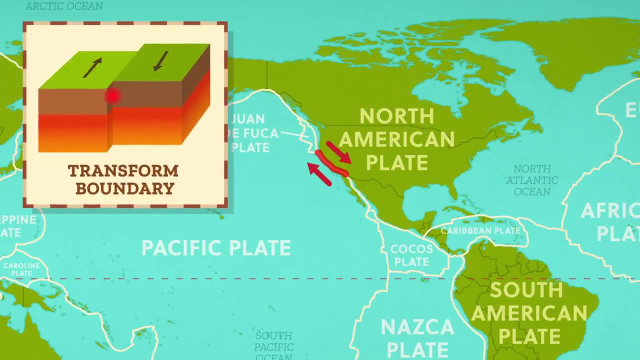 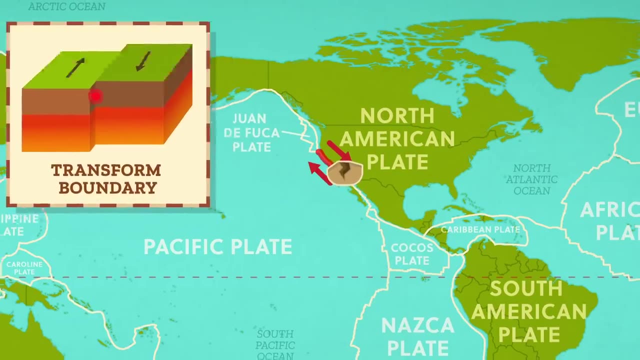 Where the plates touch they can get stuck and stress builds up. as the rest of the plate continues to move. The stress causes the rocks to break suddenly, lurching the plates forward and causing earthquakes. So plates are moving away from each other, moving towards each other and sliding past. each other. But there's one more type of boundary that's not very common along the Ring of Fire. When continental crust converges with oceanic crust, The ocean crust usually gets subducted. But when two continental plates collide, neither plate is subducted. 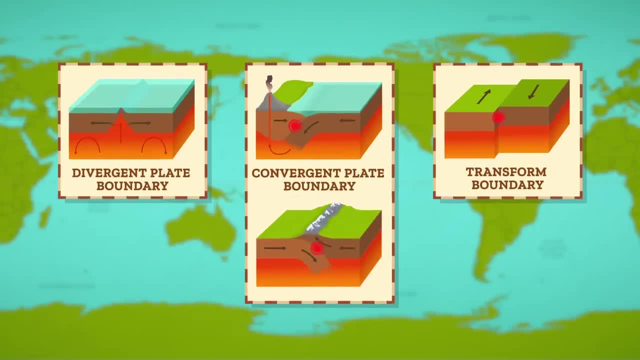 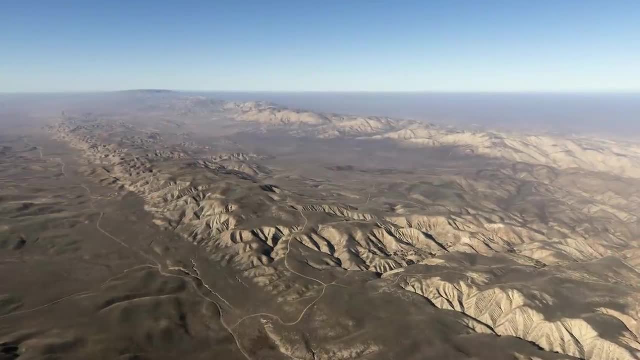 The collision compresses the crust, folding and pushing up huge mountain ranges Like the Himalayas. They sit where the Indian Plate is converging with the Eurasian Plate. So even as we speak, the structure of the Earth is changing as plates move all over. 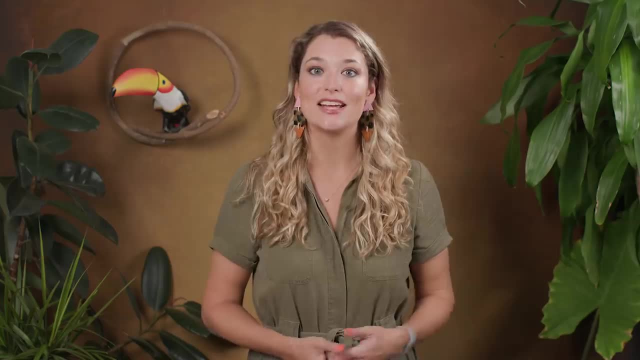 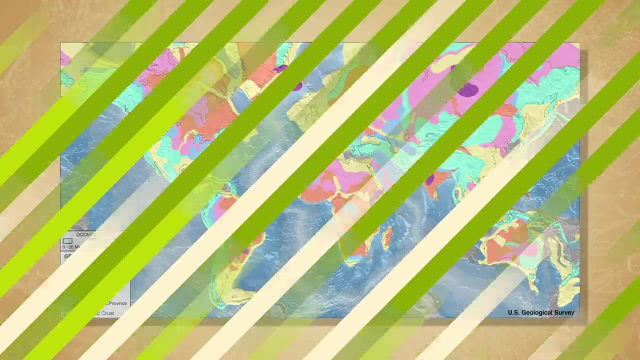 the world In the years following the Revolution. the plate tectonics theory has been fine-tuned And while we know a lot about how new ocean floor is created, how land masses form is also still being debated. We think continents grow from a nucleus of ancient and stable, igneous and metamorphic. 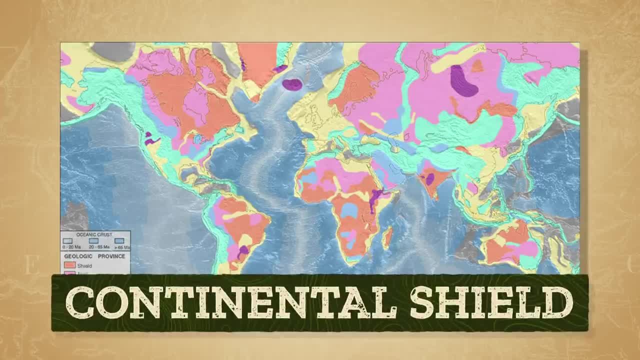 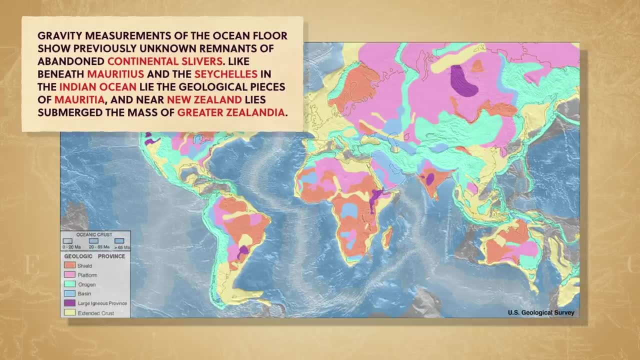 rocks And where these rocks are exposed at the surface is called a continental shield, And fragments of the crust that might originally have been offshore island arcs, undersea volcanoes or islands like New Zealand or Madagascar are added to the main continent by collision. 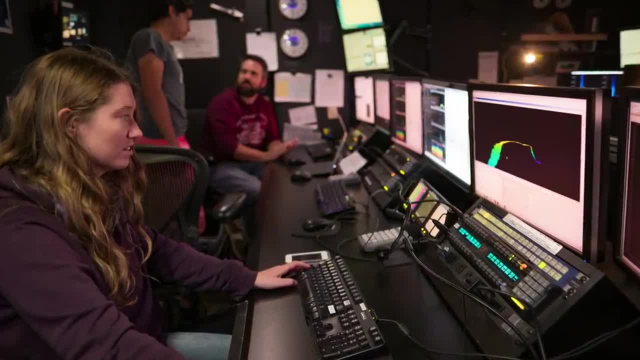 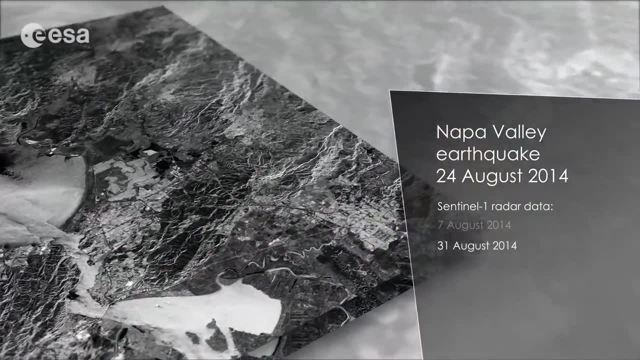 Today, in 2021, we continue to explore plate tectonics. Plate motion is detected by satellites like the European Sentinel series, which record changes in Earth's surface down to the millimeter. The story of fragmented, linear and non-magnetic Earth's surface can be found on the Earth's 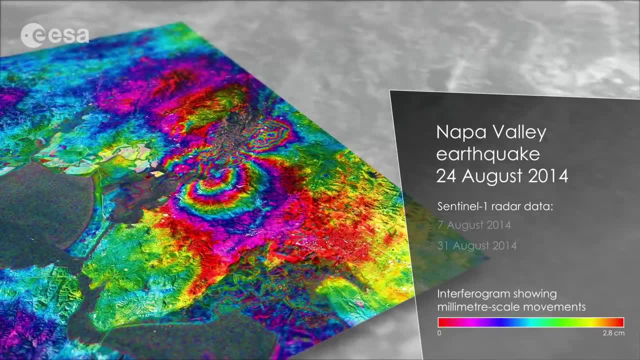 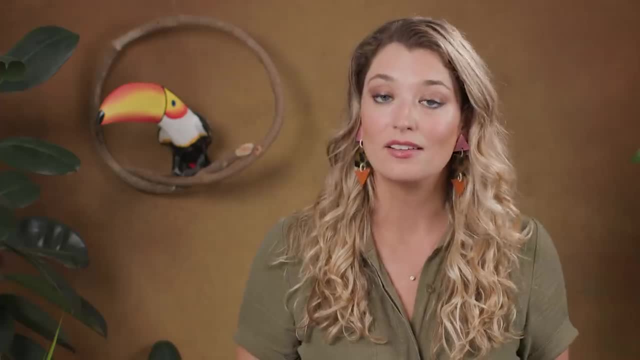 surface. The fact that fragmented lithospheric plates moving around Earth's surface has had many twists and turns, But it's not over. Scientists want to know what caused the outer shell to crack apart in the first place and how the recycling of the crust began.